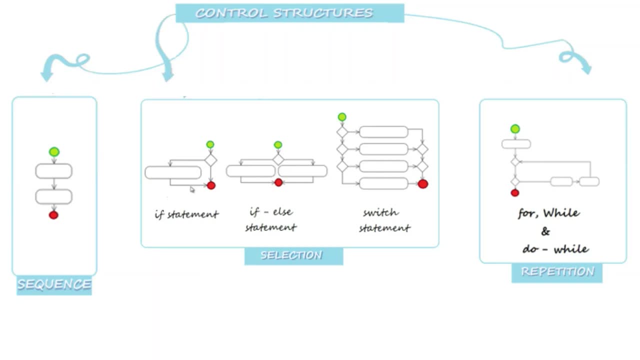 of our programs as boxes of various kinds, and their order is shown by connecting the boxes with arrows. The green and red boxes represent our start and stop points respectively, and we will be using such charts when planning out how we write our codes and are going to create our programs. 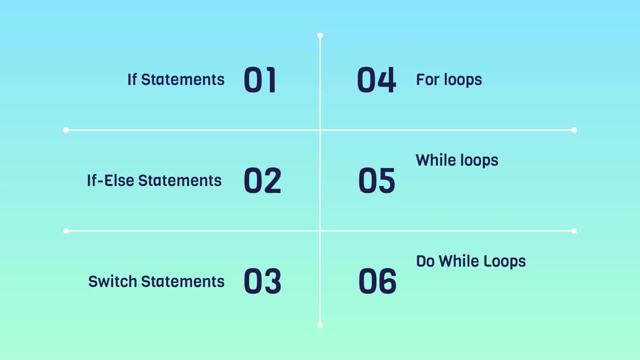 We will be giving coding examples of the four of the six implementations of selection-repetition control structures that you can use in your own programs. For more information about the while and do-while loops, refer to my video on AP Computer Science, A playlist called While vs Do-While Loops. 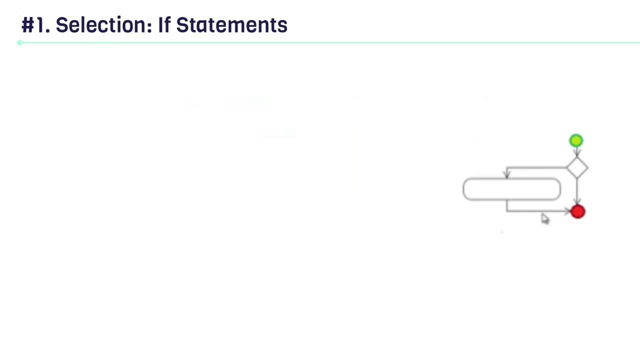 An if statement is a programming conditional statement that, if proved true, performs a function or displays information. In the example provided, if the value of x were equal to any number less than 10, the program displays hello world when the script is run. However, if our 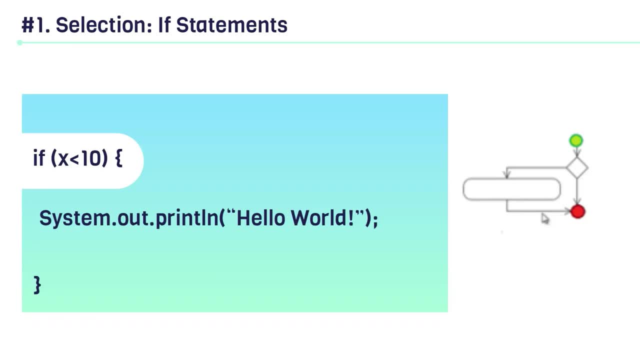 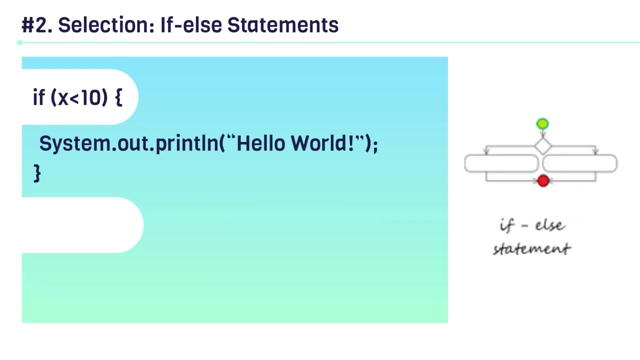 value of x is equal to or greater than 10, then nothing will happen, since we did not fit the conditional statement, and so we skip to the end of our program. Now let's say we actually want something to happen when that condition is not met. This is where an if-else statement comes into. 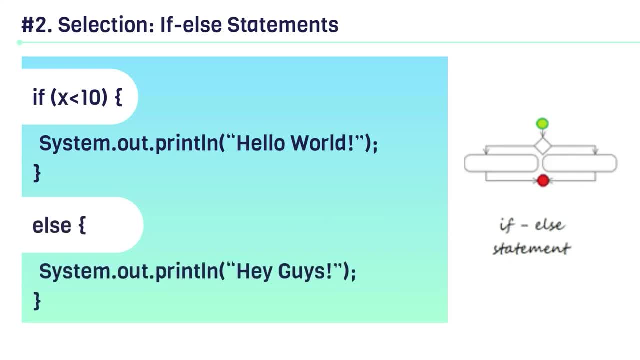 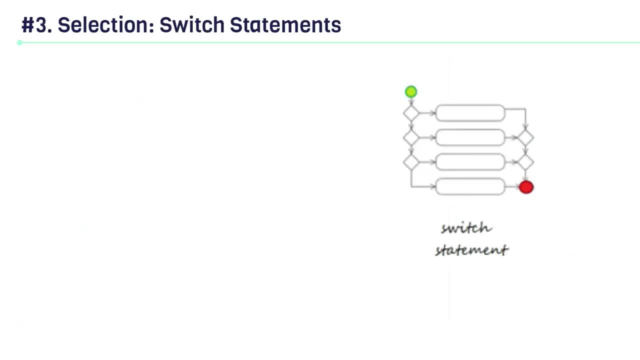 play. Therefore, if our value does not equal to 10, then we get kicked out of the initial if statement and move onto our else statement to print out hey guys instead of hello world. But let's say we have a lot of if-else statements that we want to use various conditions that must: 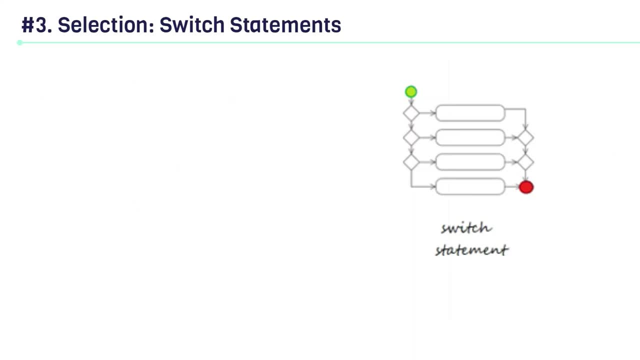 be met and even more possibilities of what we can output. This would be the case if we have an if-else statement. This is where switch statements come into play. Switch case statements are a substitute for long if statements that compare a variable to several. 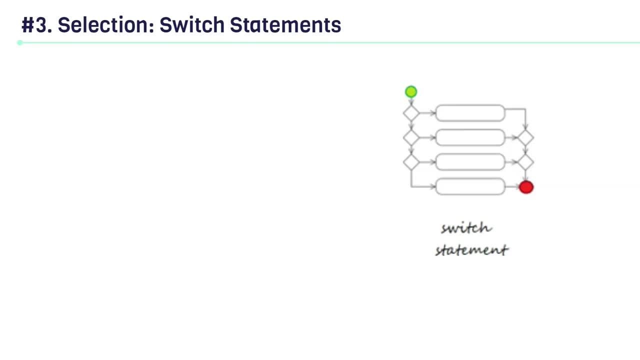 integral values. The switch statement is a multi-way branch statement providing an easy way to dispatch execution to different parts of code based on the value of the expression. For example, let's say that we want to see what day of the week it is based off of a number. 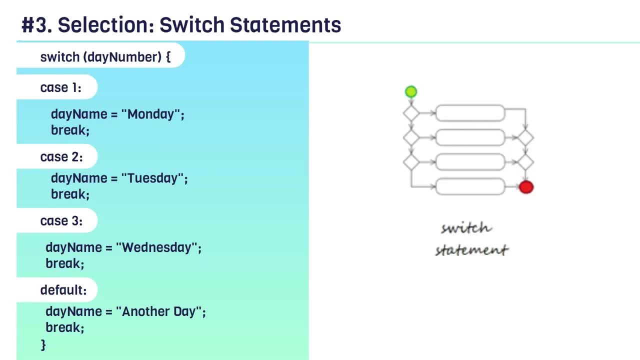 If our integer day number is equal to 1,, then we match case 1, and so our day name is Monday and we break out of the switch statement. If the integer is 2,, then it matches case 2, day name is Tuesday, and so on If our day number doesn't match any of our cases. 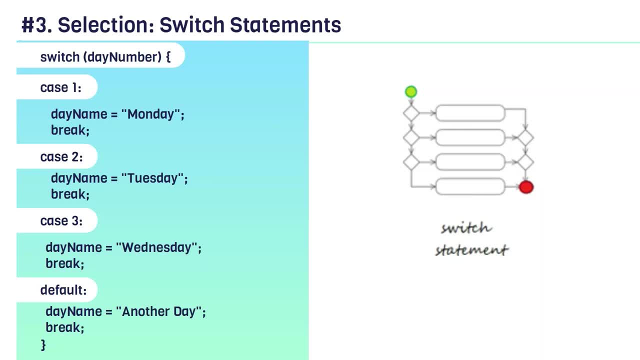 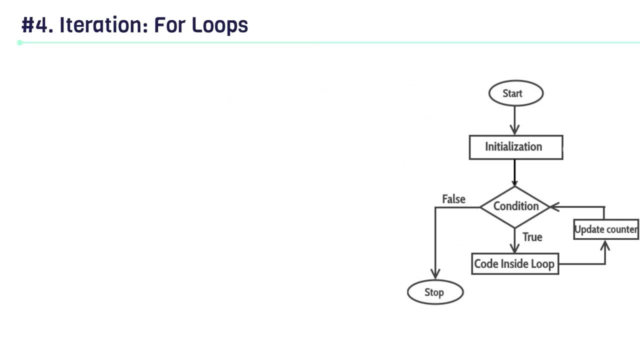 then we resort to our default value of another day and break out of the switch statement. Now onto our iterative or repetitive control structures. Here we will only talk about for loops, which allow our code to be executed repeatedly. A for loop has two parts: a header specifying the iteration.